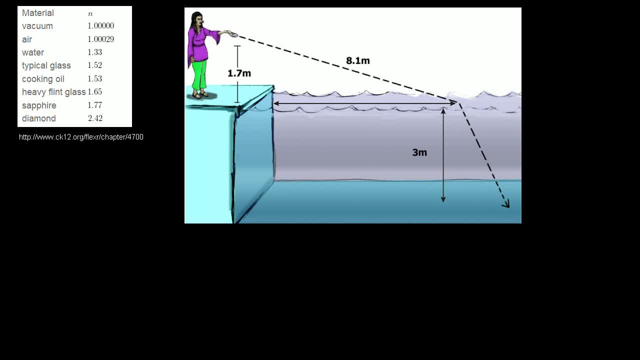 Let's do a slightly more involved Snell's Law example. So I have this person over here sitting at the edge of this pool And they have a little laser pointer in their hand And they shine their laser pointer. So in their hand, where they shine, 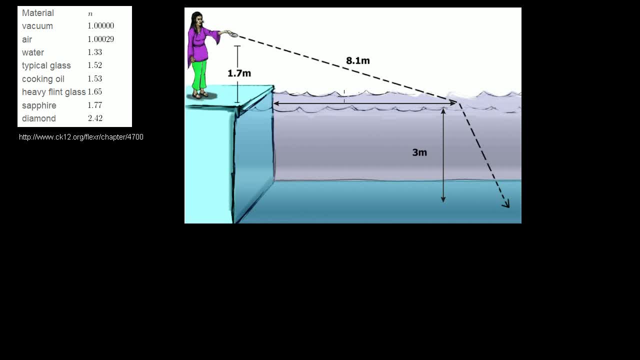 it's 1.7 meters above the surface of the pool And they shine it. so it travels 8.1 meters to touch the surface of the water And then the light gets reflected inwards, going to a slower medium If you think about the car analogy. 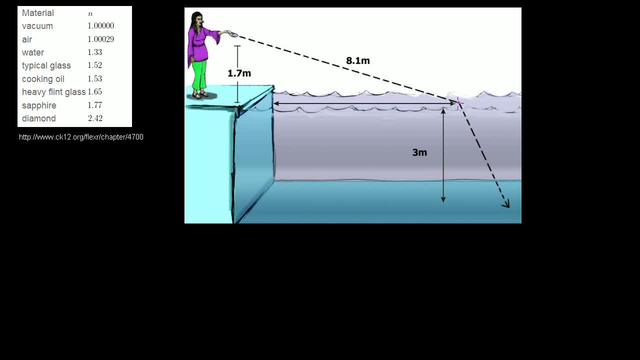 the outside tires get to stay outside a little bit longer, So they move faster, So it gets refracted inward And then it hits the bottom of the pool at some point right over here, And the pool, they tell us, is 3 meters deep. 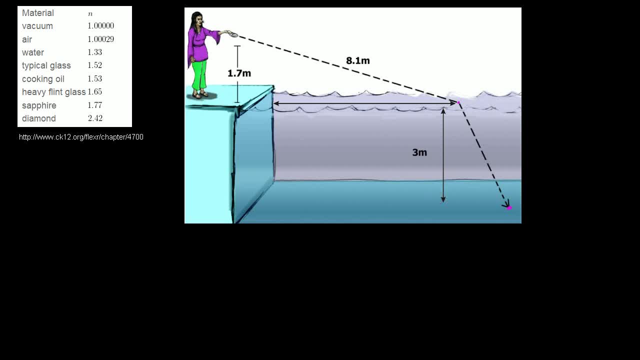 What I want to figure out is: how far away does this point hit? So what is this distance right over here? What is this distance right over there? And to figure that out, I just need to figure out what this distance is. I need to figure out what this distance is. 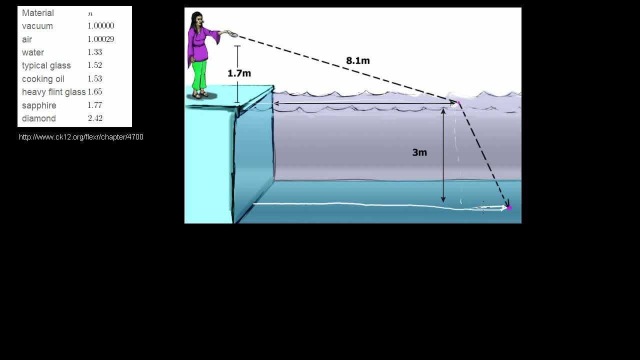 So this distance right over here, And then figure out what that distance is And then add them up So I can figure out this part. I'm trying to do it a different color, This part, right until we hit the surface of the water. 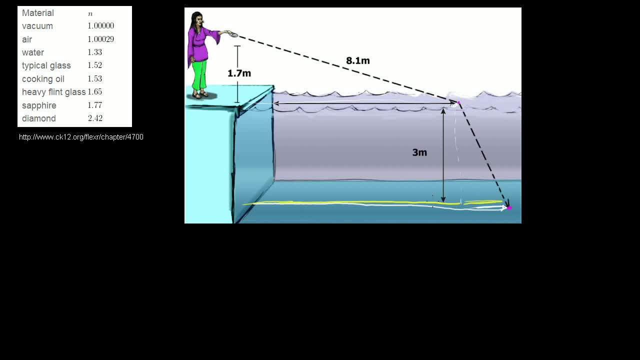 And then figure out this incremental distance just like that, And hopefully, with a little trigonometry and maybe a little bit of Snell's law, we'll be able to get there. So let's start on maybe what's the simplest thing. 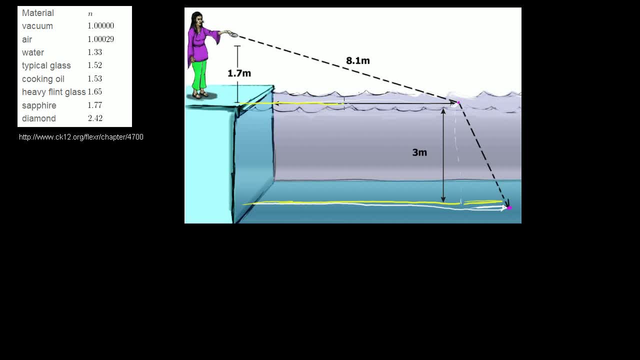 Let's just figure out this distance, And it looks like it will pay off later on As well. So let's figure out this distance right over here. So just the distance along the water, the surface of the water, to where the laser point actually. 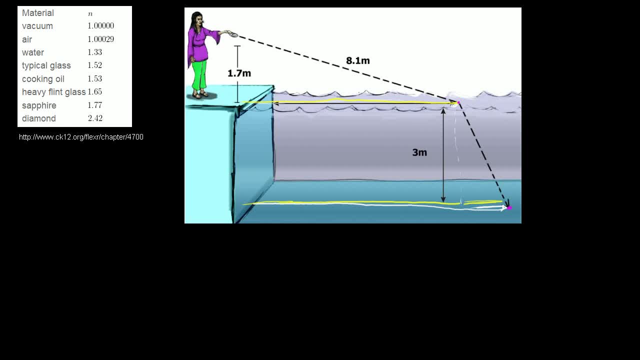 starts touching the water, And this is just a straight up Pythagorean theorem problem. This is a right angle, This is the hypotenuse over here. So this distance, let's call this distance x, x squared plus 1.7 meters squared. 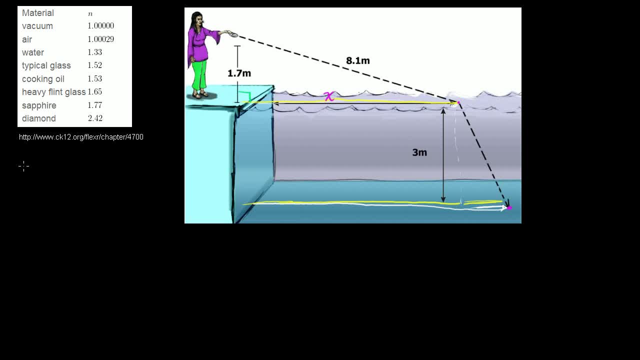 is going to be equal to 8.1 squared. Just straight up Pythagorean theorem, Plus 1.7 squared is going to be equal to 8.1 squared. Or we could subtract 1.7 squared from both sides. 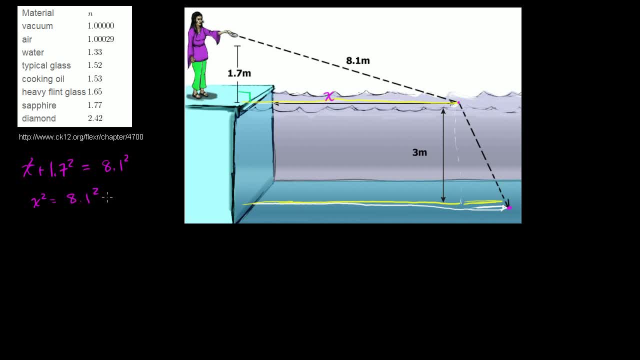 We get: x squared is equal to 8.1 squared minus 1.7 squared. If we want to solve for x, x is going to be the positive square root of this, Because we only care about positive distances. x is going to be equal to the principal root of 8.1 squared. 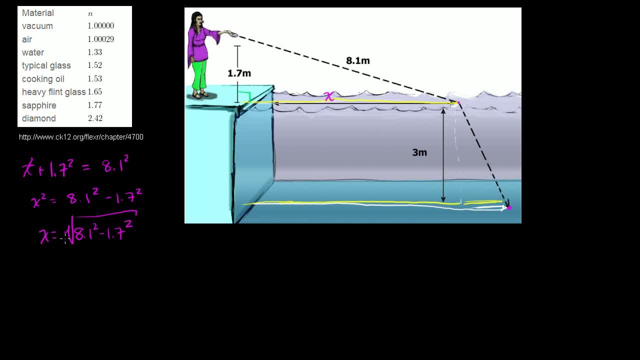 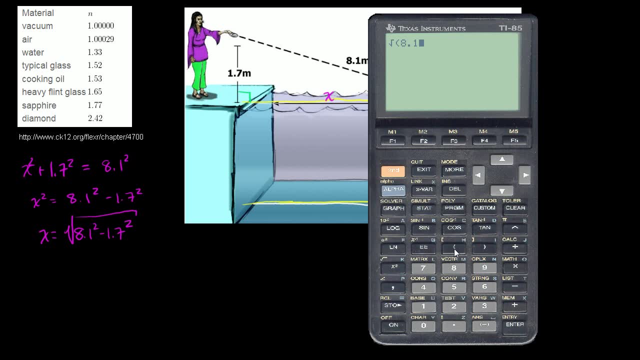 minus 1.7 squared. And let's get our calculator out. So x is going to be equal to the square root of 8.1 squared minus 1.7 squared And I get 7.92.. So x is about 7.92.. 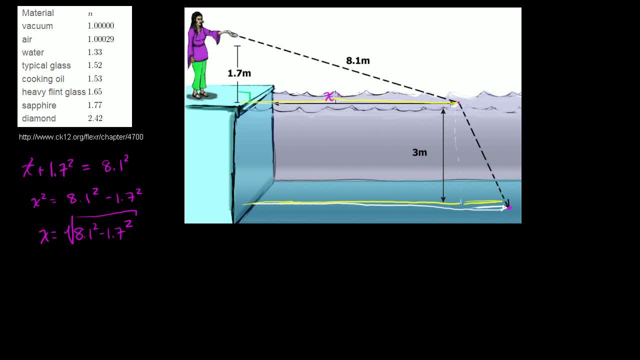 Although we could save that number there so we can get a more exact number. So this is equal to 7.92.. That is x. Now we just have to figure out this incremental distance right over here, add that to this x and then we know this entire distance. 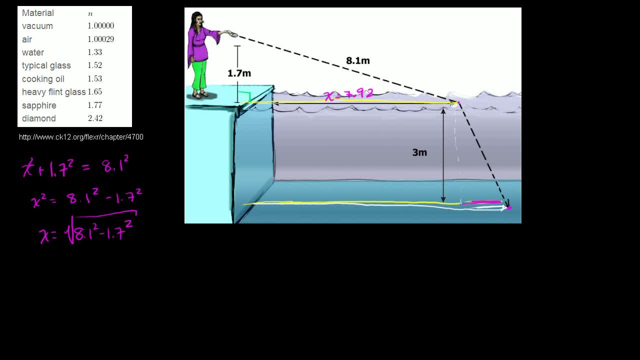 So let's see how we can think about it. So let's think about what the incident angle is, and then the angle of refraction is. So I've dropped a perpendicular to the interface or to the surface. So our incident angle is this angle right over here. 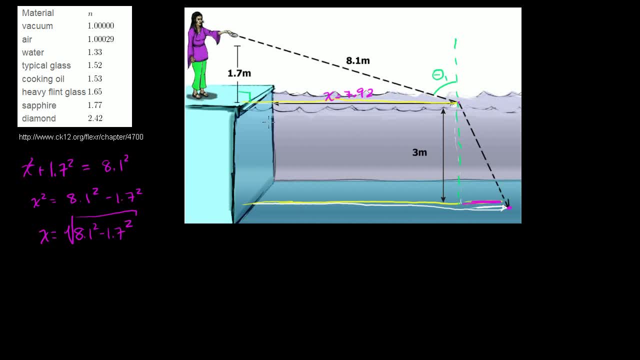 That is our incident angle. And remember Snell's law. we care about the sine of this angle. Actually, let me just write down what we want to care about. So we know this is our incident angle, This is our angle of refraction. 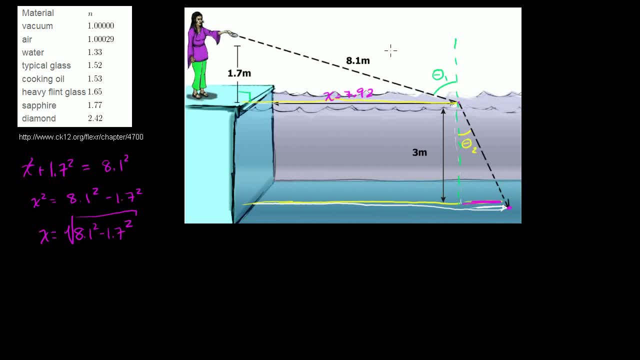 We know that the index of refraction for this medium out here- and this is air, So the index of refraction for air times, the sine of theta 1.. This is just Snell's law Times, our incident angle right here- is going to be equal to the index of refraction. 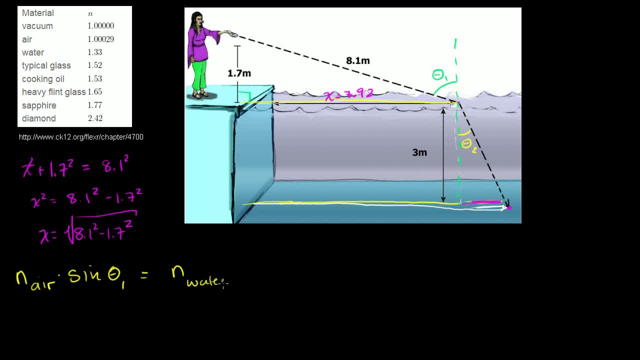 for the water and we'll put the values in at the next step. times the sine of theta 2.. Times the sine of our refraction angle, sine of theta 2.. Now we know we can figure out these ends from this table. 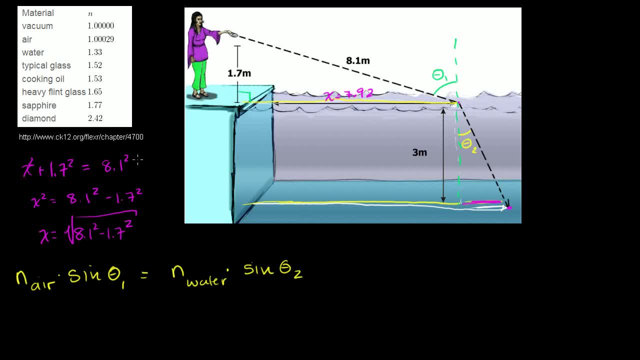 right over here. I actually got this problem from ck12.org's flexbook as well, or at least the image for the problem, And so If we want to solve for theta 2, or if we know theta 2,, we can then solve for this. 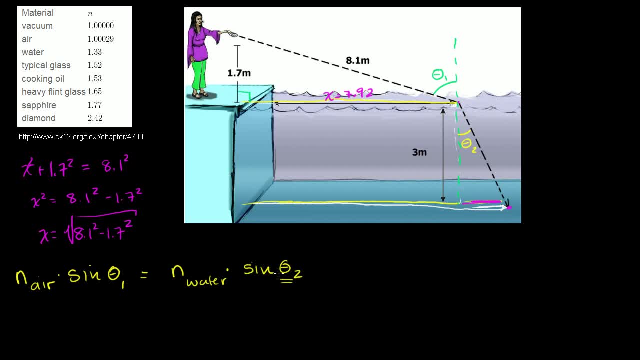 And we'll do that with a little bit of trigonometry. Actually, we won't even have to. If we know the sine of theta 2, we'll be able to solve for this. All right, well, we'll think about either way. 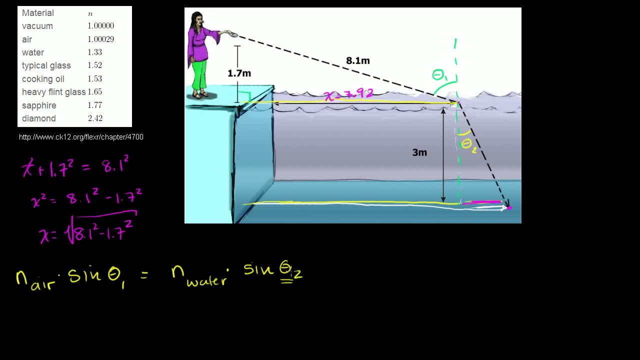 Actually we'll just solve for this angle And then if we know this angle, then we'll be able to use a little trigonometry to figure out this distance over here. So to solve for that angle we can look up these two. 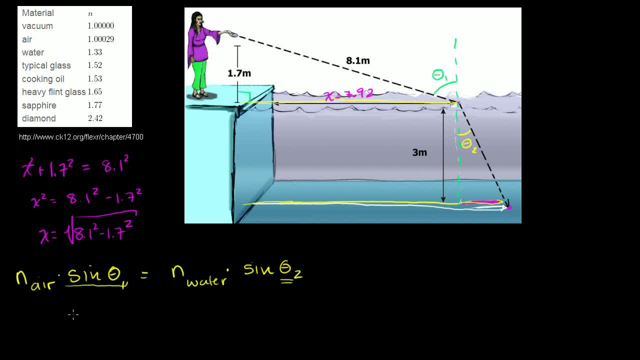 And so we just have to figure out what this is. We need to figure out what the sine of theta 1 is. So let's put in all of the values. Our index of refraction of error is 1.00029.. So let me put that in there. 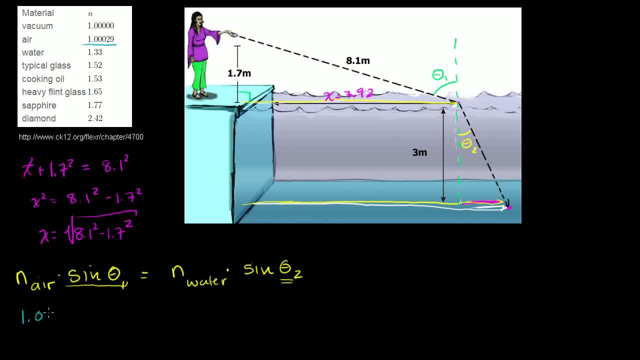 So that's this 1.00029.. So 1.00029 times the sine of theta. And you say, oh, how do we figure out sine of theta? We don't even know what that angle is. But remember, this is basic trigonometry. 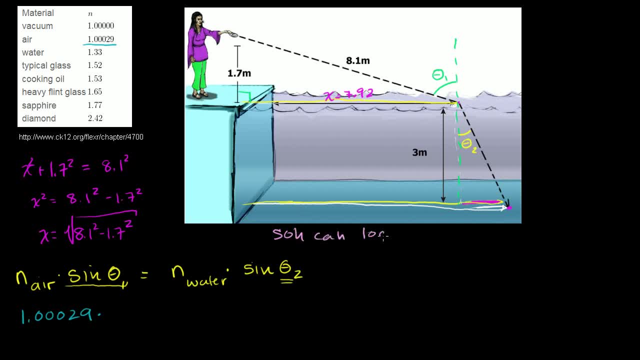 Remember SOH CAH TOA Sine is opposite of our hypotenuse. So if you have this angle here, let's make it part of a right triangle. So if you make that as part of a right triangle, Opposite over hypotenuse, 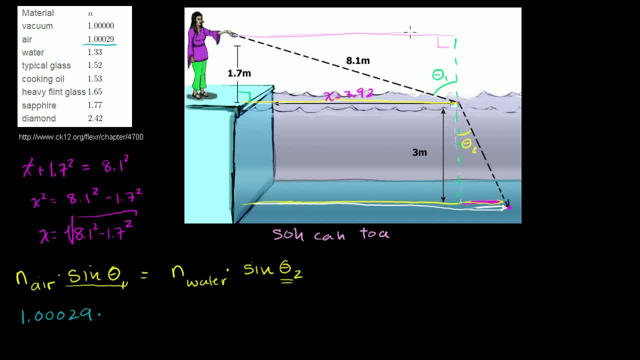 It's the ratio of this side, It's the ratio of that distance to the hypotenuse. This distance over here we just figured out, It's the same as this distance down here, It's x. So this is 7.92.. 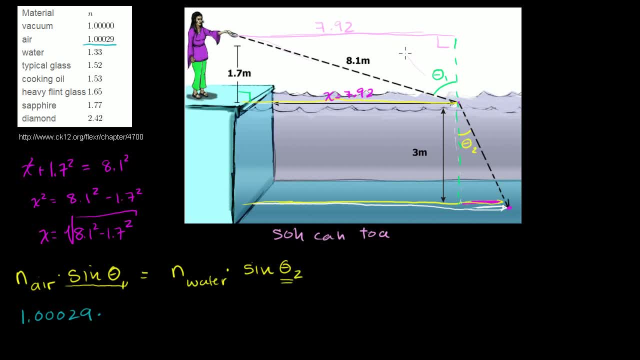 So the sine of theta 1 is going to be the opposite of the angle opposite over the hypotenuse. That just comes from the definition of sine. So it's going to be times. So this part right over here: sine of theta 1.. 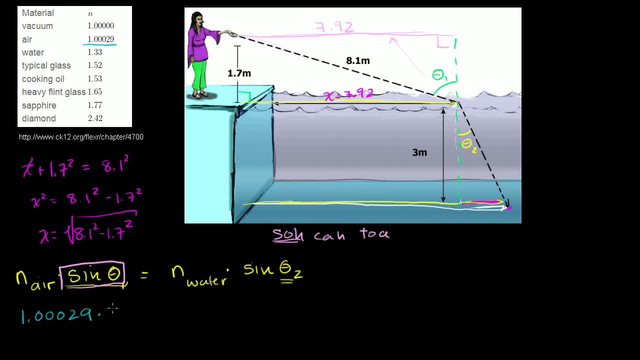 We don't even have to know what theta 1 is. It's going to be 7.92 over 8.1.. And that's going to be equal to the index of refraction of water. So that's index over 1.33.. 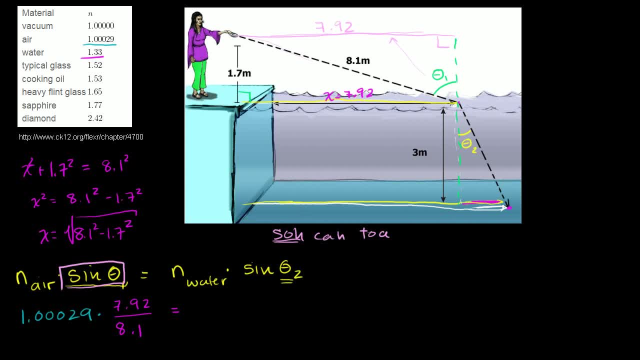 So let me do that in a different color, So that's going to be 10.. Now I wanted to do a different color, So that's going to be: let me do it in this dark blue, So it's going to be 1.33 times sine of theta 2.. 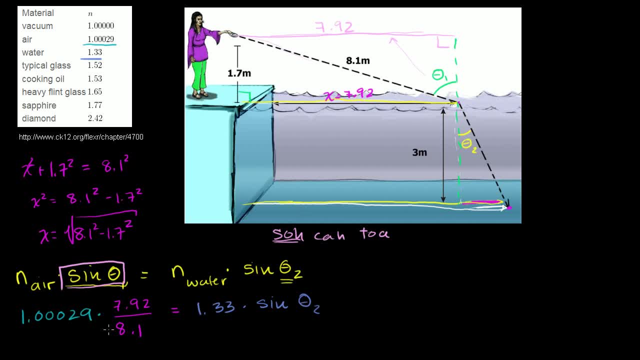 And so if we want to solve for sine of theta 2, you just divide both sides of this equation by 1.33.. So let's do that, So I'll do it over here. So if you divide both sides by 1.33, we get 1.00029 times 7.92.. 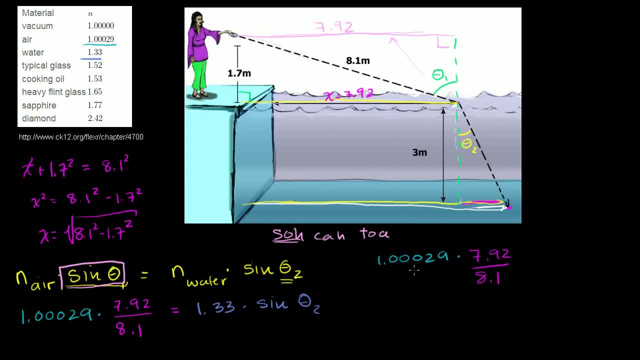 And we're also going to divide by 1.33.. So we're also dividing by 1.33.. That is going to be equal to this sine of theta 2.. That is going to be equal to sine of theta 2.. 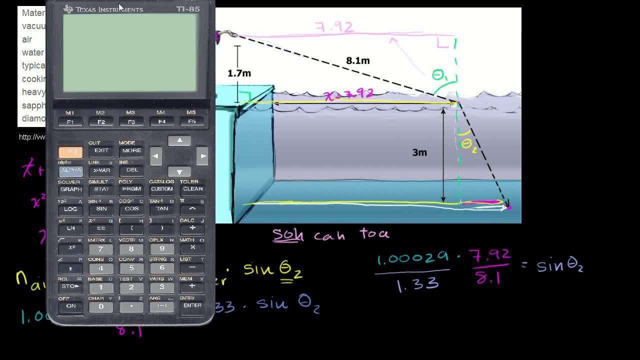 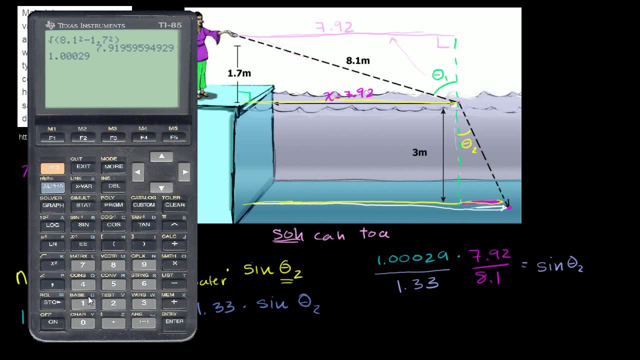 So let's figure what that is. So let's do that, Get the calculator out. Let's get the calculator out. So we have 1.00029 times 7.92.. So that's 1.00029.. And we're also going to divide by 1.33.. 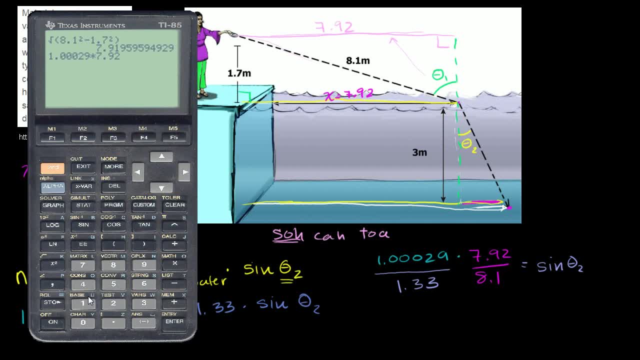 So let's do that, Get the calculator out. So that's 1.00029 times 7.92.. Well, actually I could even say times. second answer: if we want this exact value, That was the last sum to do that. 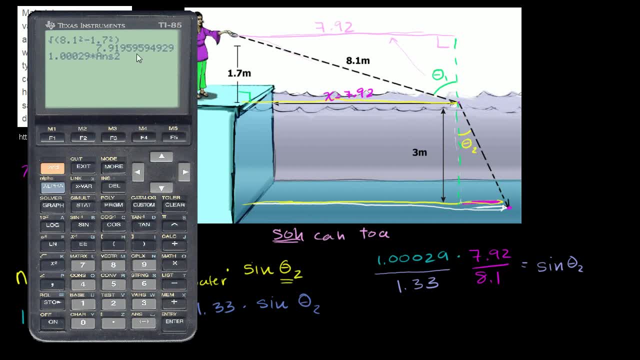 Second answer: So that's the actual precise, not even rounding. And then we want to divide by 1.33.. That's this right here. And then we want to divide by 8.1. And we get that And that's going to be equal to the sine of theta 2.. 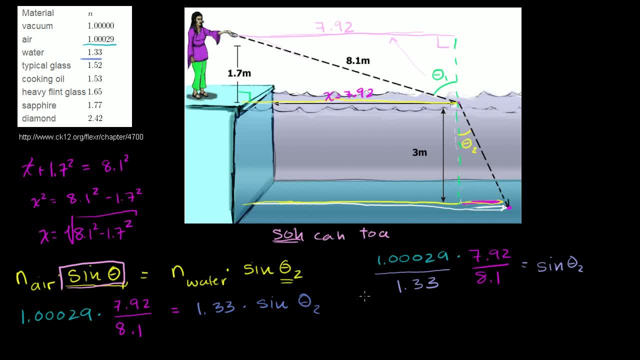 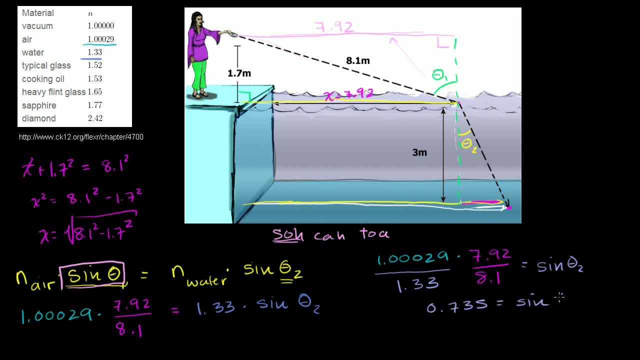 735 is equal to the sine of theta 2.. Now we could take the inverse sine of both sides of this equation to solve for theta 2.. So we get theta 2 is equal to. let's just take the inverse sine of this value. 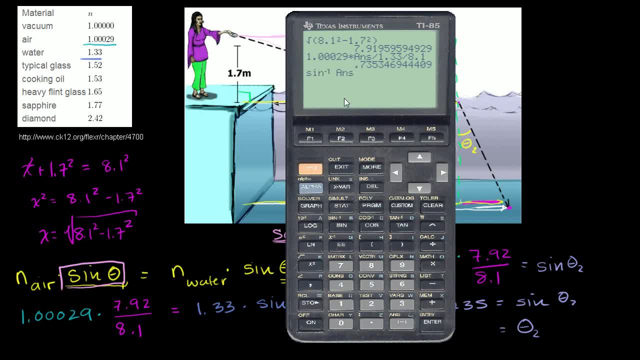 So I take the inverse sine of the value that we just had. So answer is just our last answer And we have theta 2 being 47.3, let's say around 0.34 degrees. So this is 47.3.. 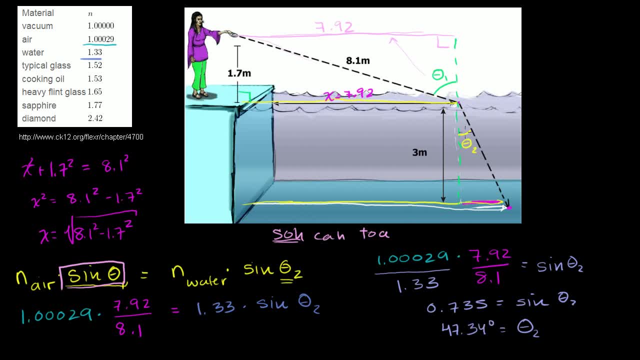 47.34 degrees. So we were able to figure out what theta 2 is- 47.34 degrees. So now we just have to use a little bit of trigonometry to actually figure out this distance over here, Now what trig ratio involves. so we know this angle we want. 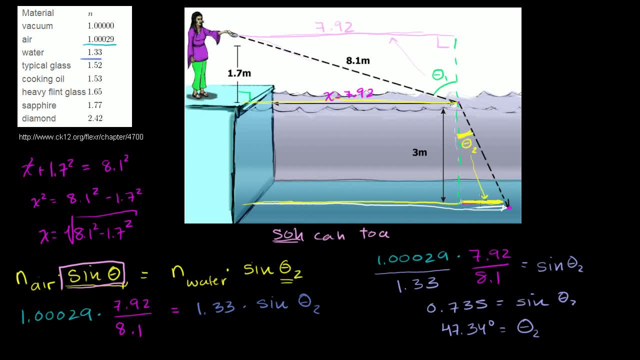 to figure out its opposite side. we want to figure out the opposite side to that angle and we know the adjacent side. We know that this, right here, is 3.. So what trig identity deals with opposite and adjacent? Well, tangent, TOA. 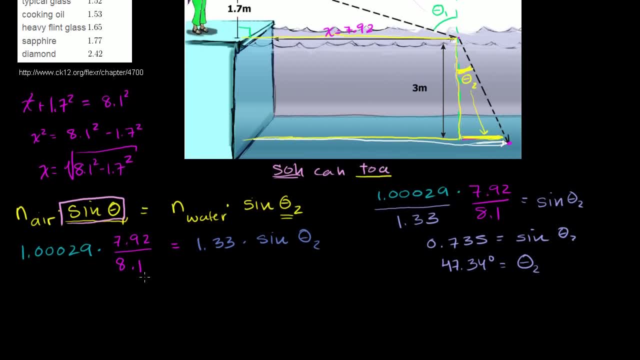 Tangent is opposite over adjacent, So we know that the tangent of this angle right over here of 47.34 degrees is going to be equal to this opposite side over here. So let me just call that. I'll call that y. 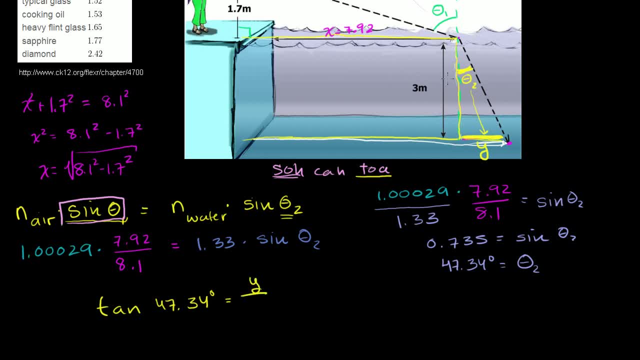 It's going to equal y over our adjacent side, and that's just 3 meters. Or if we want to solve for y, Or if we want to solve for y, we multiply both sides of this equation by 3. You get 3 times. the tangent of 47.34 degrees is equal to y. 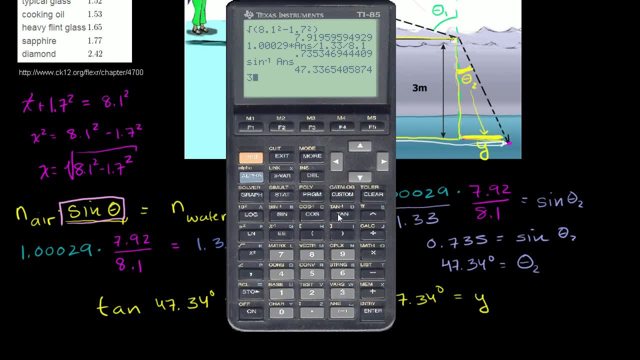 So let's just get the calculator out. So 3 times the tangent of that, 47.34 degrees. I'll use the exact answer: 3 times the tangent of that is 3.255.. So this distance right here y. 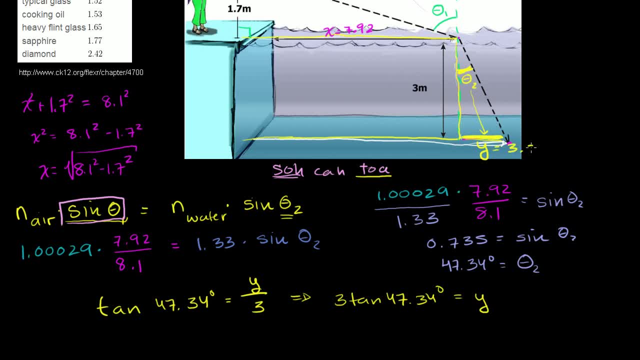 And we're at the home stretch. y is equal to 3.255 meters. Now our question was: what is this total distance? So it's going to be this distance: x plus y plus the 3.25.. So x was 7.92.. 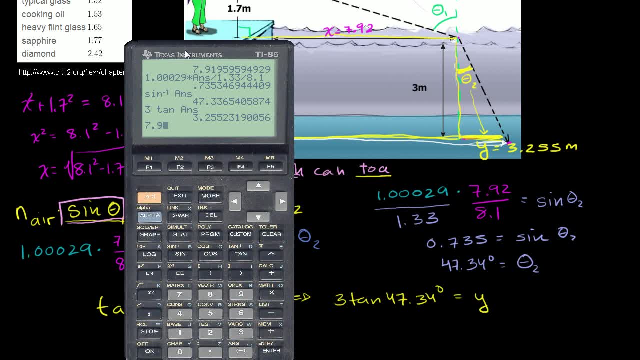 And I'll round here. So it's literally just going to be 7.92 plus our answer just now, plus our answer right now. So we get about 11.18.. Or maybe, if we want to really round or get the same number of significant, 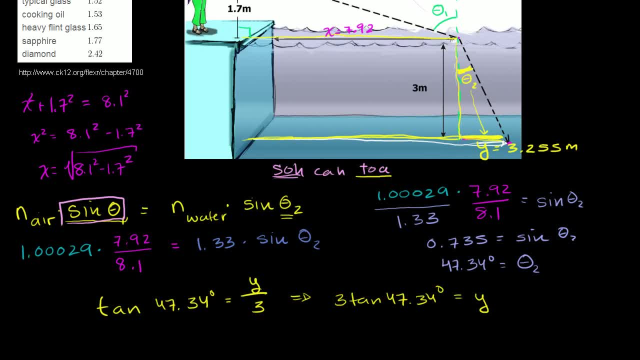 digits that we started maybe 11.2 meters. I'll just say 11.18 meters. So this right here is the distance that we wanted to figure out is the point on the bottom of the pool where the actual laser pointer actually hits the surface of the pool. 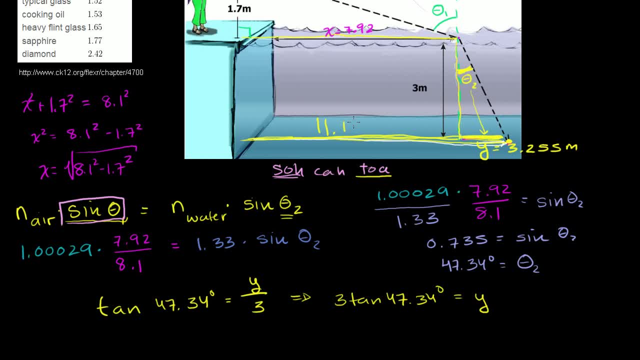 will be 11.18 approximately. I'm rounding a little bit Meters, Meters from this edge of the pool right there. Anyway, hopefully you found that useful. It was a little bit more involved of a Snell's Law problem.